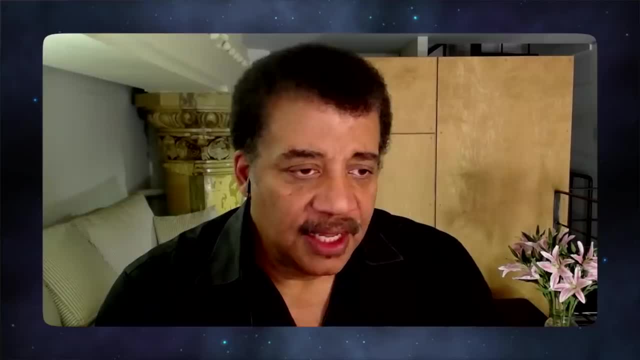 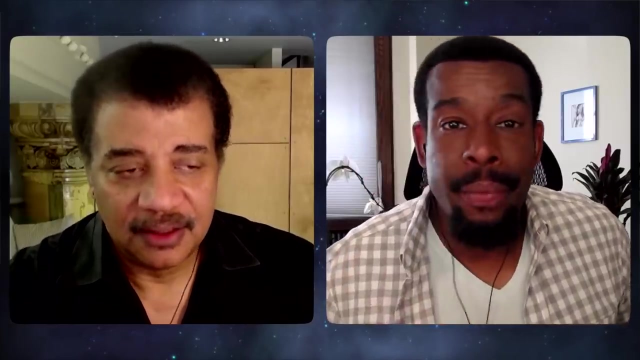 me out. You got to hear me out, okay. Okay, I, as an astrophysicist, know that we have something called color temperature. okay, I am aware of that. We practically invented that concept. okay, Well, I like photography, so that's how I know color temperature. Well, I'm going to get there. 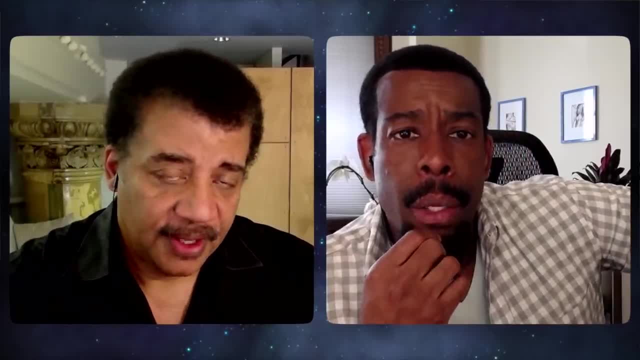 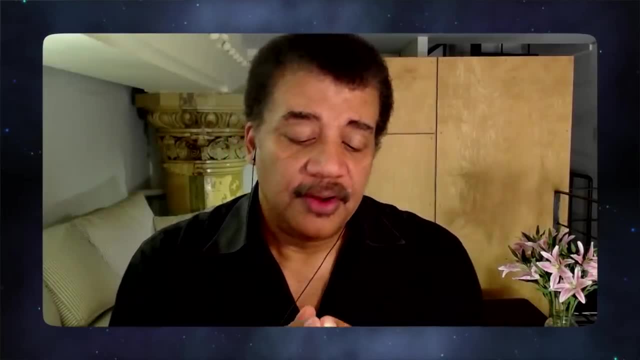 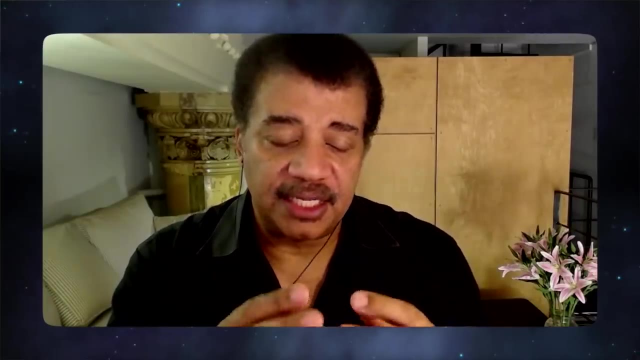 and you're going to find out why I have issues. okay, Uh-oh. So here's what happens If you have an object that is of a given temperature. if it's hotter than absolute zero, it will be radiating some electromagnetic energy. Okay, Right, So the colder it is, the longer are the 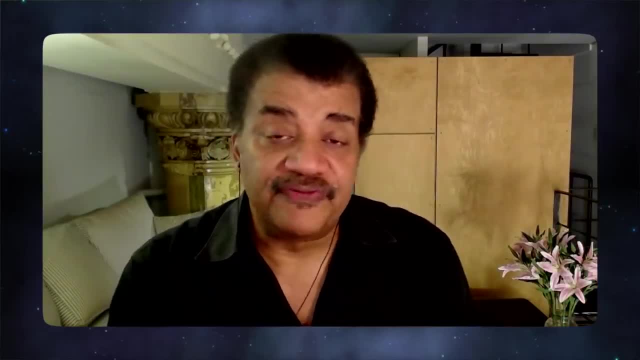 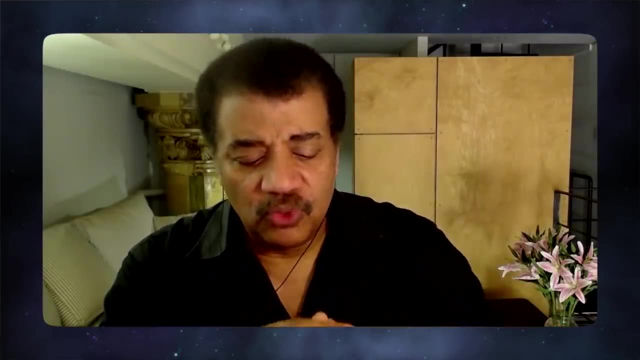 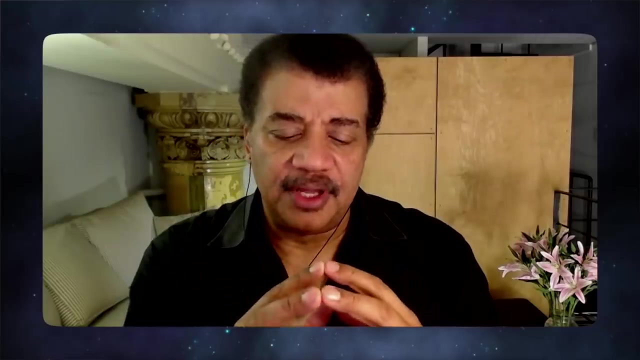 wavelengths of light. it emits radio waves. The universe is pretty cold. It's only three degrees Kelvin, that's emitting microwaves, and the hotter it gets, the more it emits light of higher and higher. Keep going. Eventually you can heat this thing up so that some of the energy that emits 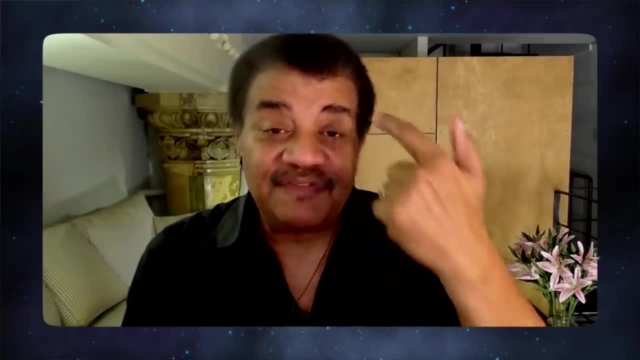 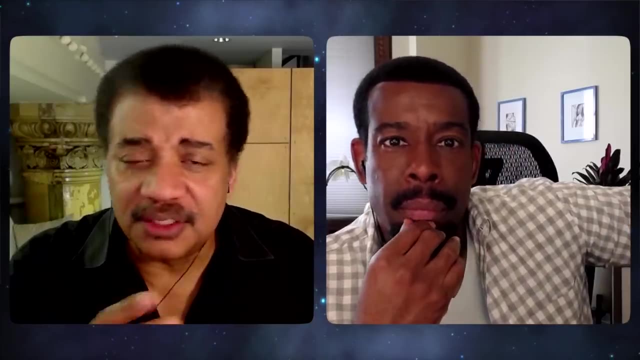 comes out in the red part of the spectrum, That object. if you looked at it with your eyes, you'd say it's red. okay, It'll start doing that at you know? 1,000, 1,500 degrees. okay, Keep increasing. 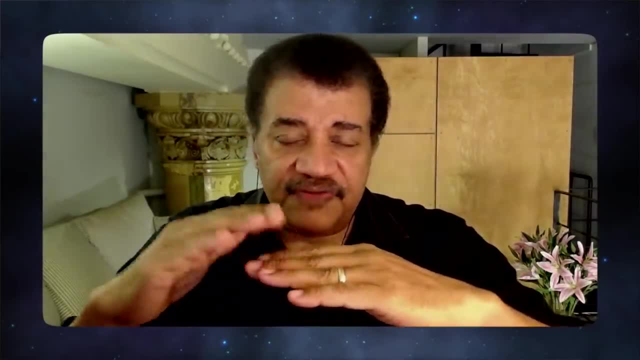 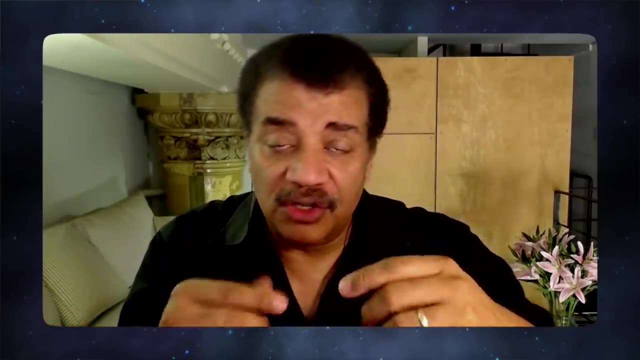 the temperature. It's not only giving you red light, it's also giving you light from the rest of the rainbow, from the rest of the optical spectrum. So it'll give you not only red, but also orange, yellow, green, blue, violet. If you do that in. 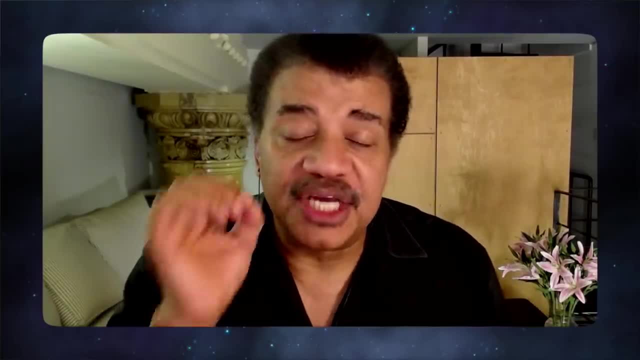 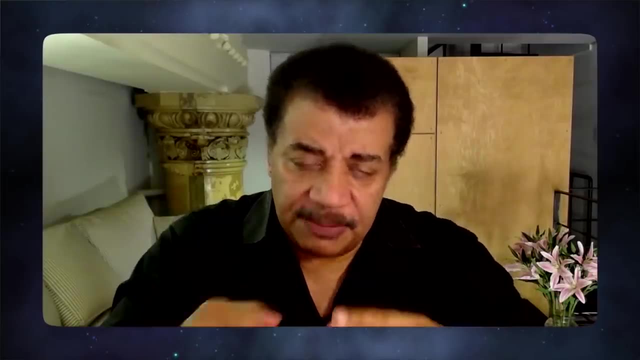 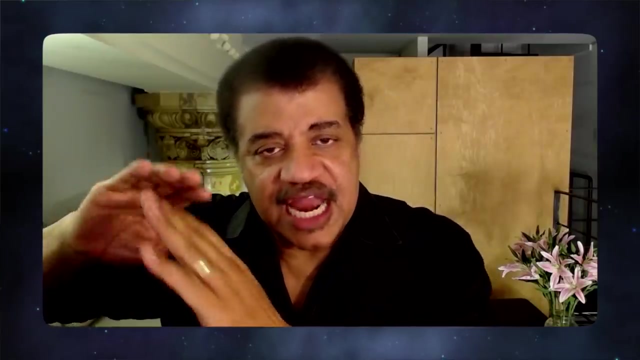 roughly equal amounts, the glowing object turns white. Okay, Because you have equal amounts of all the colors of the rainbow. So now, if you keep raising the temperature, this energy output continues to shift, and now it's emitting more blue light than red light. If you're emitting, 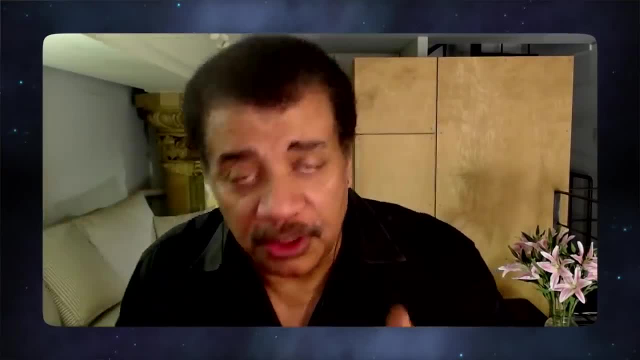 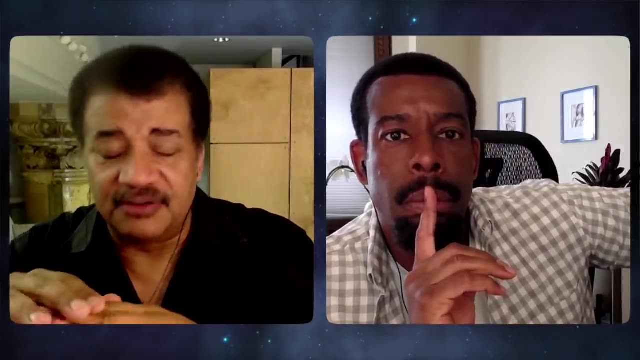 more blue than red through the spectrum, then you're emitting more blue light than red light. That object will look blue, Okay, Okay. So I'm going from like a couple of thousand degrees to like 6,000 degrees, to 10,, 12,, 15,, 20,000 degrees. Is that my on my stove? I'm getting. 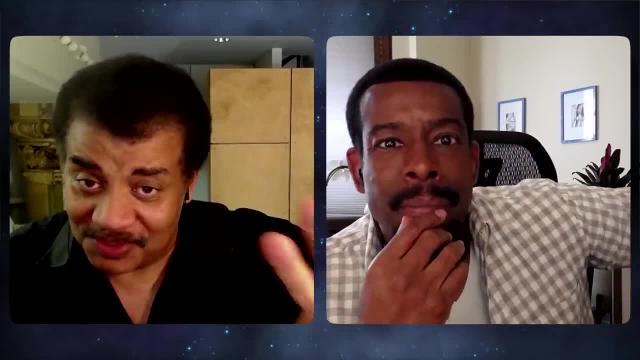 there, I'm getting there, I'm getting there. So what? Okay, I'm getting there, That's what I'm saying. That's what I'm saying, Hang with me, Hang with me. So an object goes from what is basically. 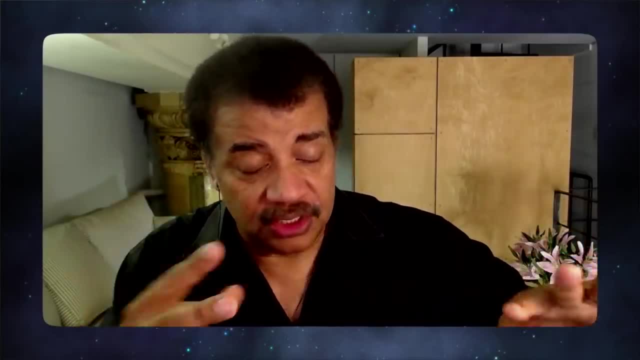 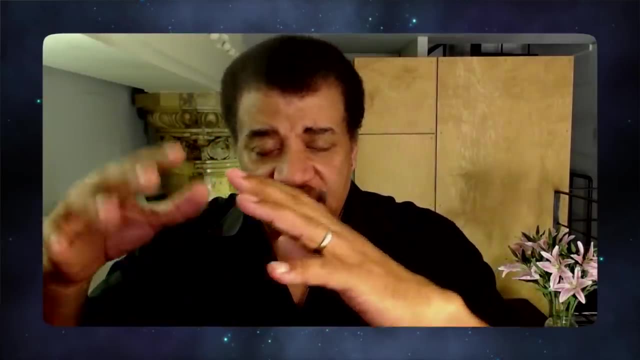 invisible to you unless you had radio wave eyeballs or microwave eyeballs- to something red and then it goes to amber and then it starts glowing white and then it'll start glowing blue and it'll forevermore glow blue, but it keeps giving you higher and higher energy It'll give. 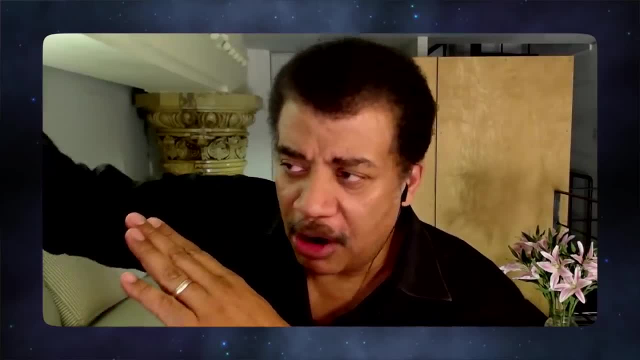 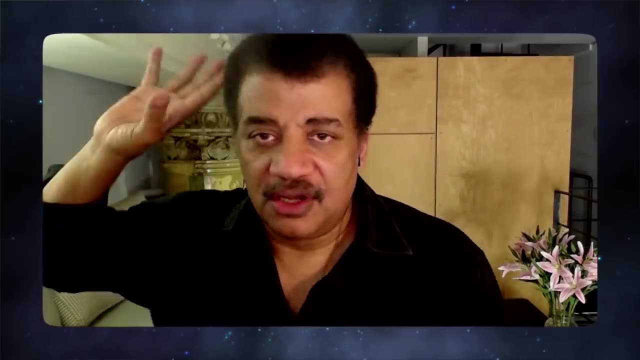 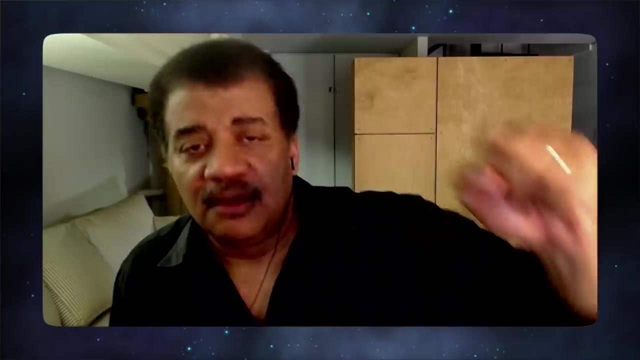 you x-rays. It can even give you gamma rays, But the part of it that comes through the spectrum is more in the red than in the blue. So hot things are blue. Medium temperature things are white. Cooler things that are still glowing are red. 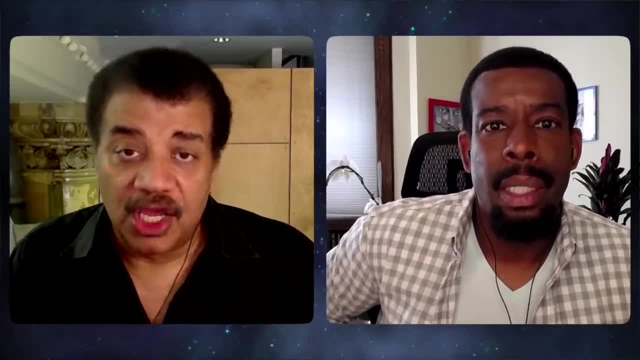 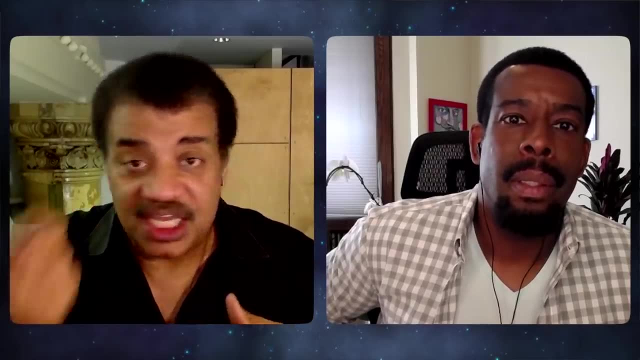 Okay. So if you have an electric stove, when you first turn it on it feels warm, but you can't see it in the dark. No, Okay, That's giving you infrared. We can't see infrared. It's got to glow. 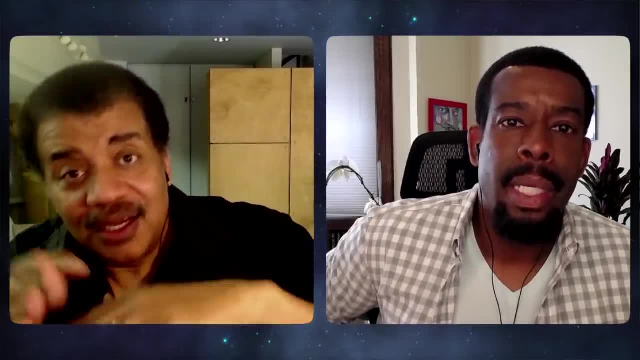 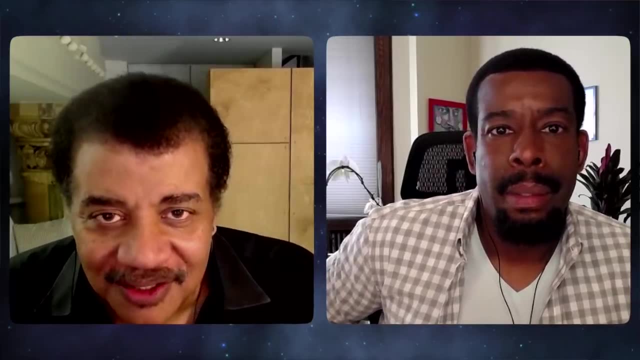 so hot that it's giving you a little bit of red Right, And then you say, oh, it's glowing red hot Right, But a red hot object is the coolest of all hots. Ah, Okay, Damn, Damn, That's what I'm. 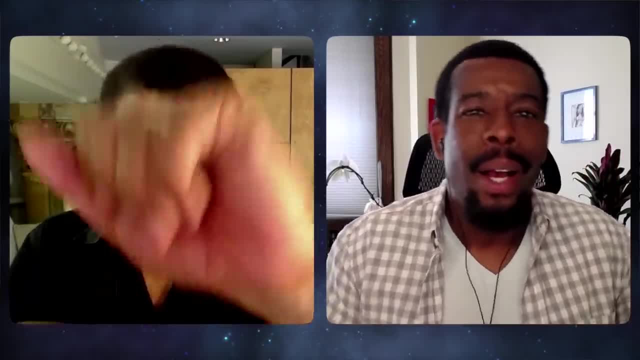 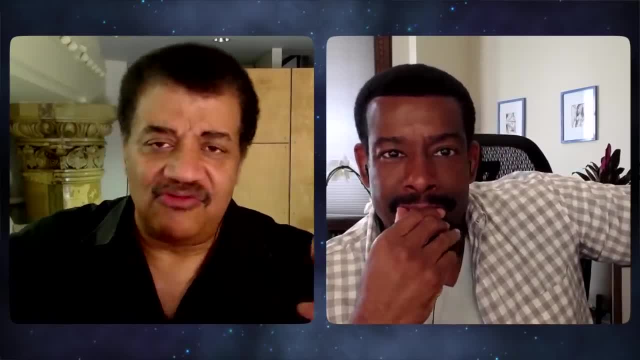 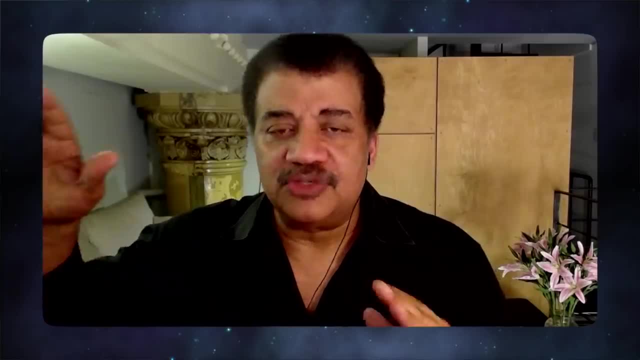 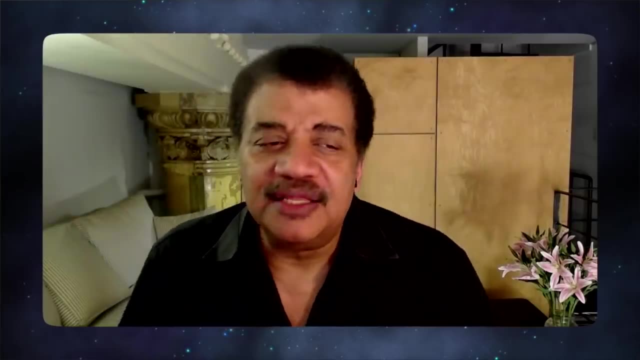 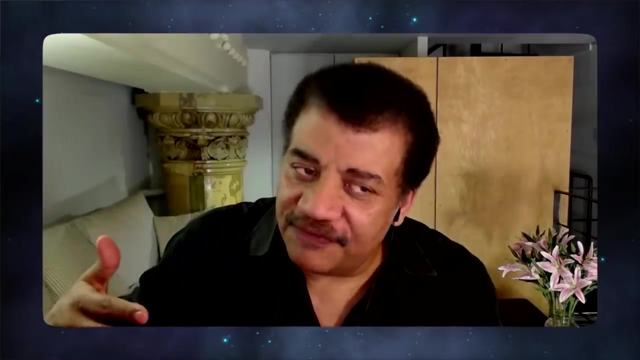 Okay, So now watch. Okay, So that is what's happening astrophysically, That's what's happening in the laws of physics, But now bring in the artistic photographer. Okay, Okay. And in art, if you're going to paint a picture, a painting, you're going to create a painting. 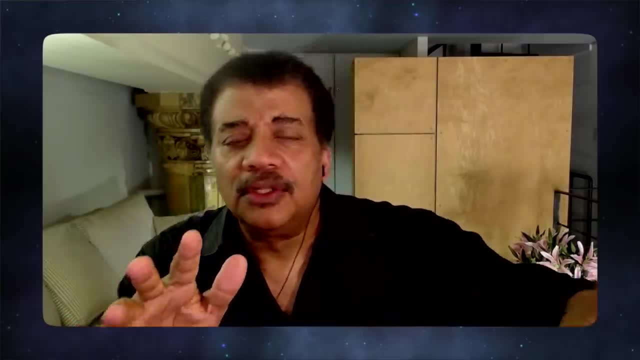 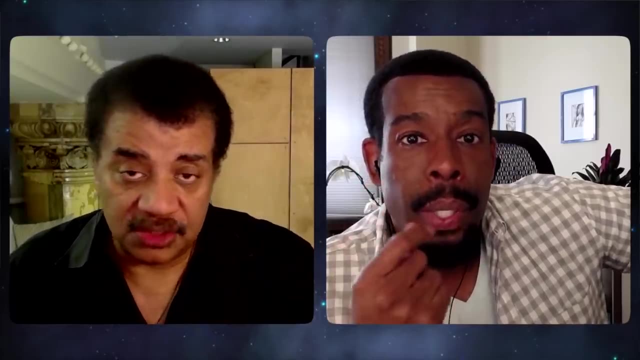 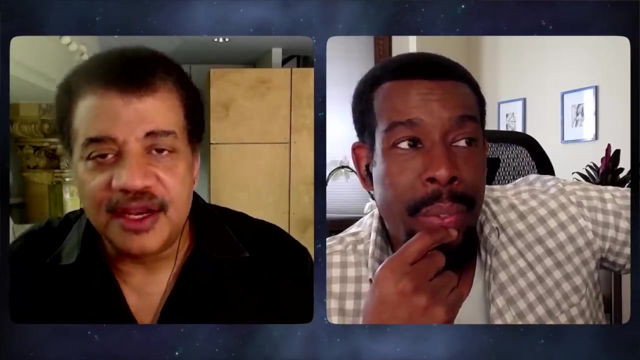 and you want the scene to feel cool like it's in the Arctic. what is your predominant color in the painting? White, White, Or not just white? Blue, Blue, Especially blue. Okay, So they say that it's cool. Right, There's a cool color, Okay. And then when they want to show something hot, 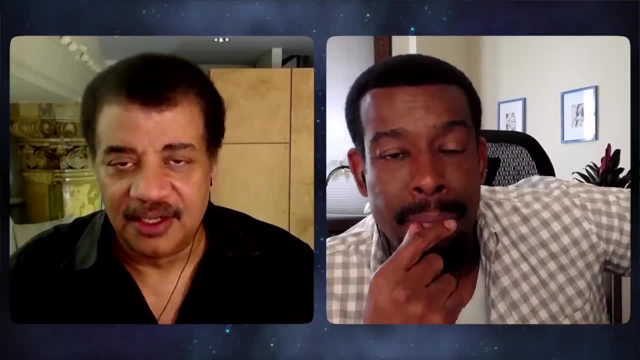 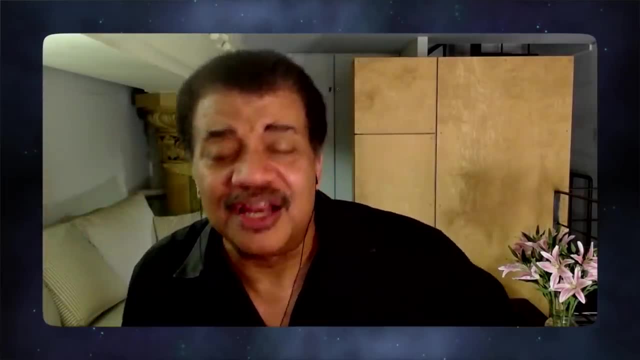 like hell and devils and everything. they use the color red. All right, Because that's how our emotions. We see ice cubes and it's bluish, And anything that got hot enough to hurt us is glowing red hot. It's rare that you'll see something so hot. 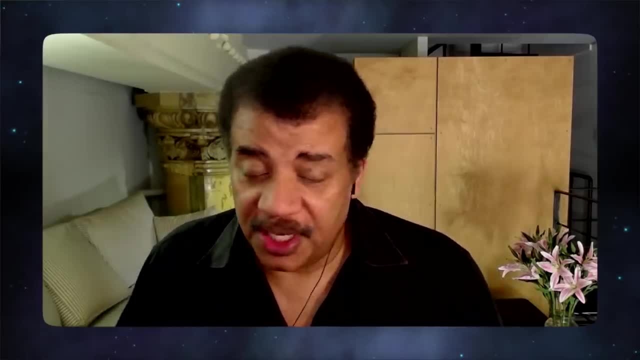 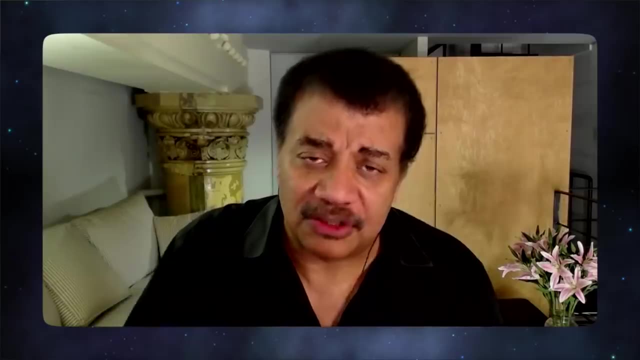 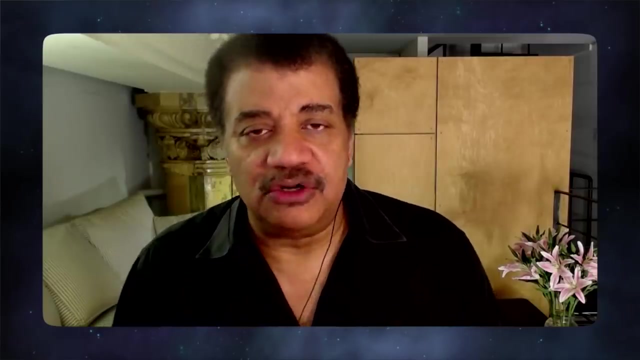 that it's glowing white or glowing blue on earth, because that stuff gets hot enough. when it's red hot, All right. So our entire life experience is shifted to the cool end of the spectrum, with us thinking that red hot is actually hot. As a result, we have the absurd. 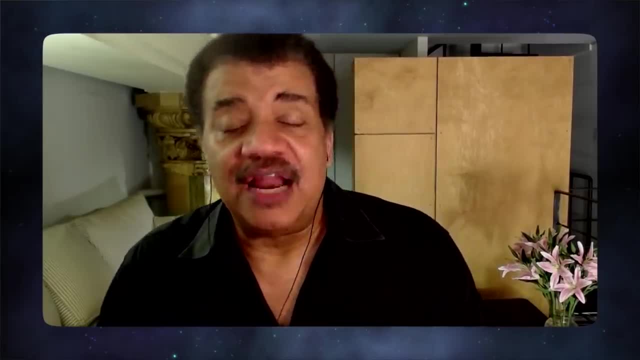 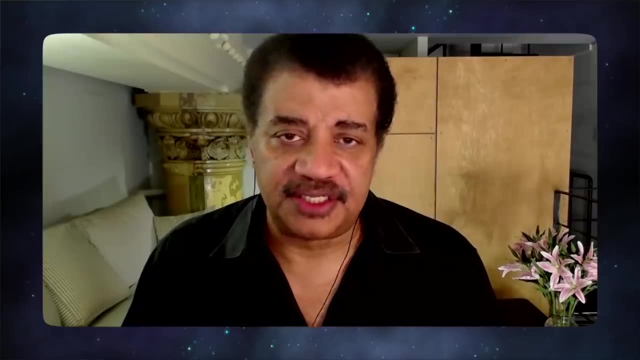 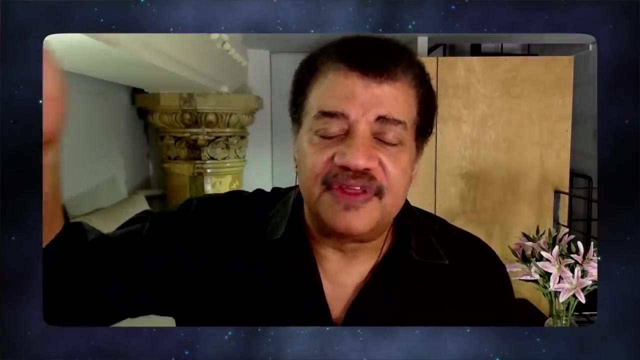 conversation between an astrophysicist and a photographer. Okay, I need a cooler lamp for this, Right. So what do they do? They get the 6,000 degree bulb instead of the 3,000 degree bulb. This is in the days when you used tungsten, but 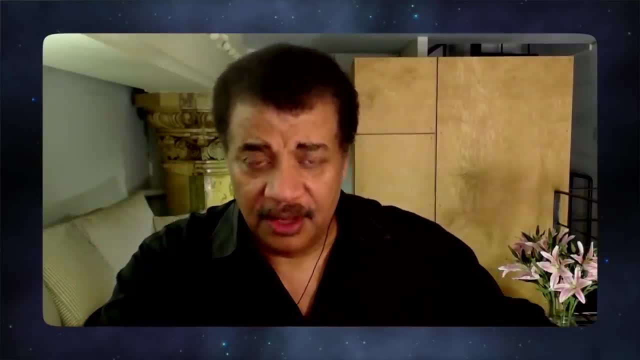 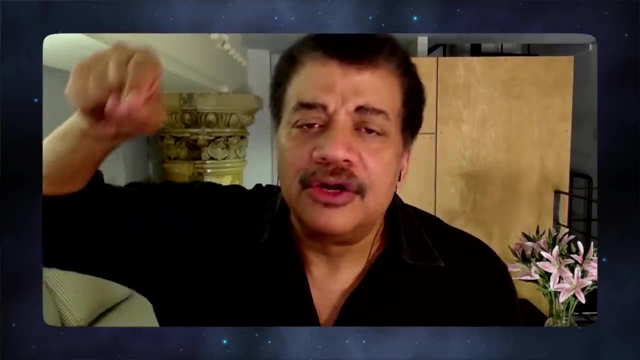 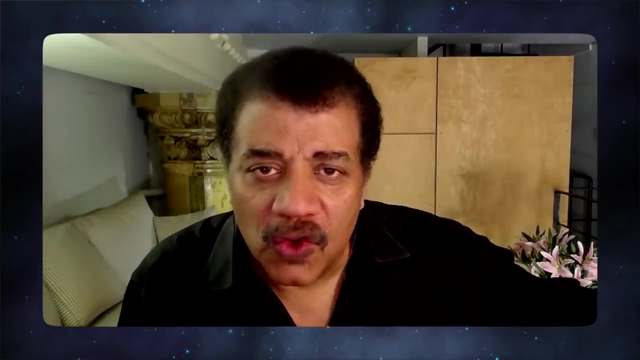 we still think of those temperatures, even in the LED world. Okay. So when they say make this scene cooler, they mean get a higher temperature lamp, And when they say we want to make this scene warmer, it means they want to put in a lower temperature lamp. that 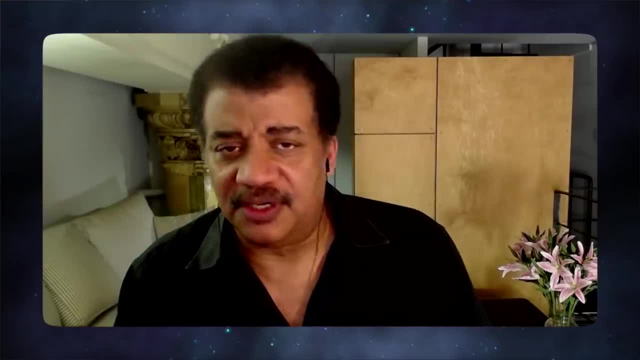 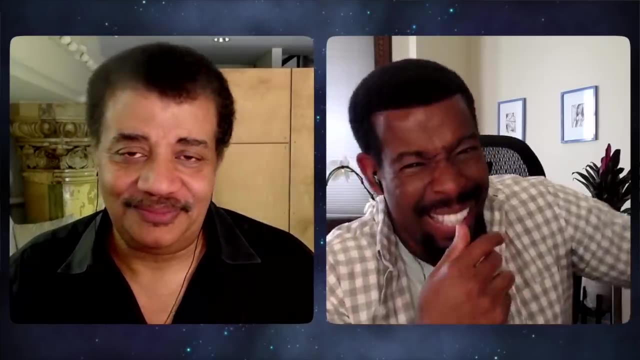 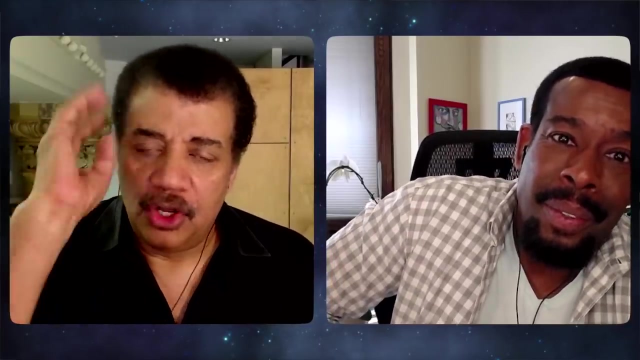 glows at like 3,000 degrees or 2,500 degrees And I'm pissed off at this. I'm just saying That's great. If you're going to be numerical about whether something is warm or cool, do you have permission to leave the article? 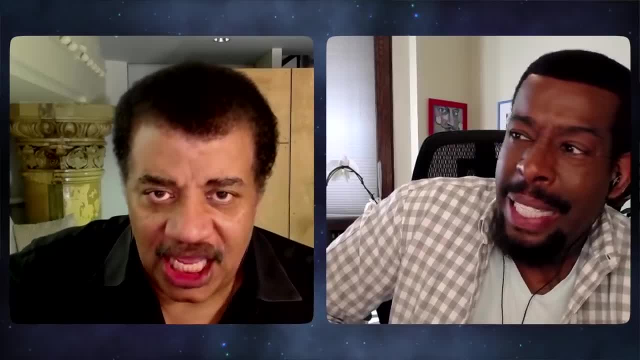 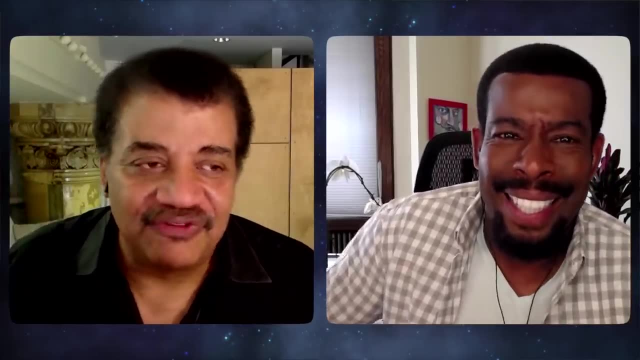 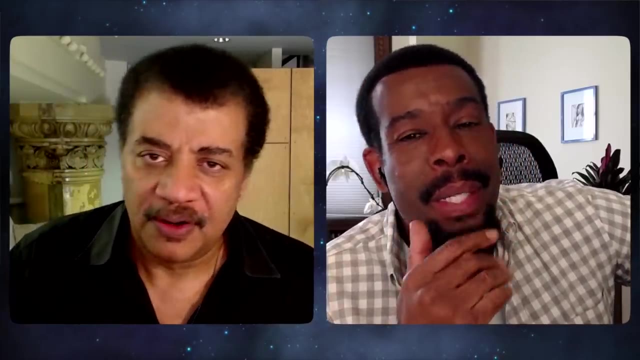 No, I'm not. I'm just saying: Well, I'm just saying if you want to say the scene is cool, blue and warm red, fine, but don't hand it a temperature, Right, Don't give it temperatures, Because you have the absurd conversation. Increase the color temperature of the lamp. 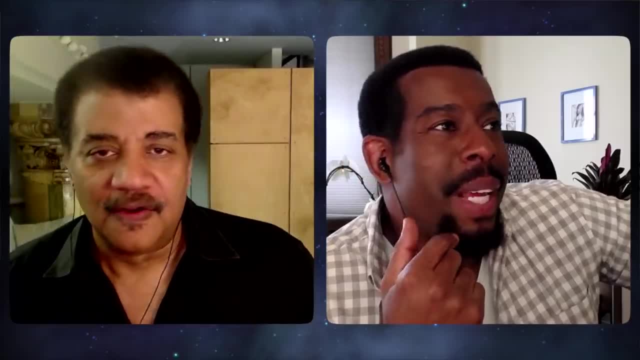 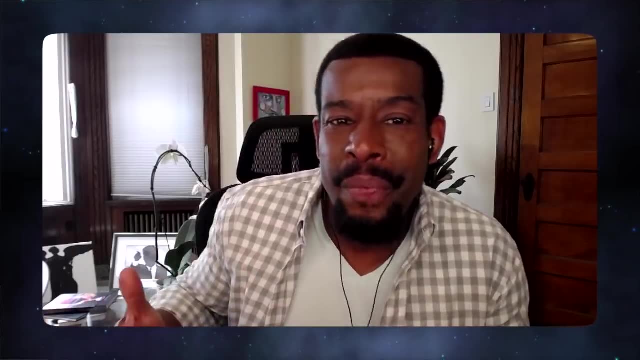 so that the scene it's illuminating is cooler. Well see, you got to do that. I hate that You have to talk to each other in temperatures. I'm not giving you that, otherwise we wouldn't know what to do. so if, if you're ever shooting something and 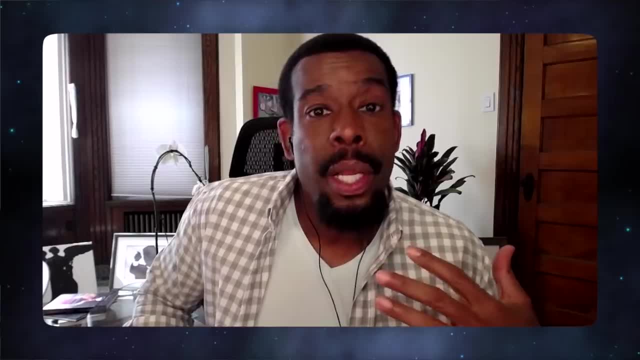 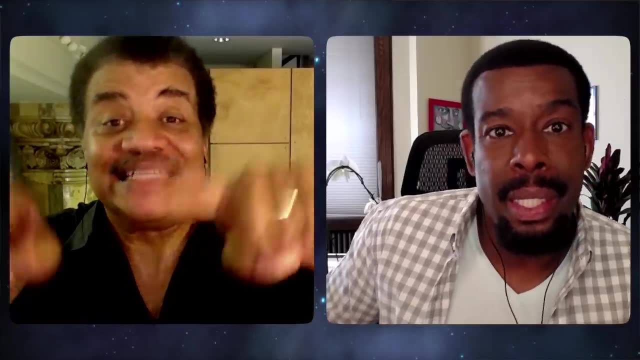 somebody says: all right, yo, let's, let's give me that, give me that daylight, and daylight is 5600. right, it's basically between that and 6,000 and, by the way, that is, that is the temperature of the Sun, right, okay, and wait, wait, wait, wait. 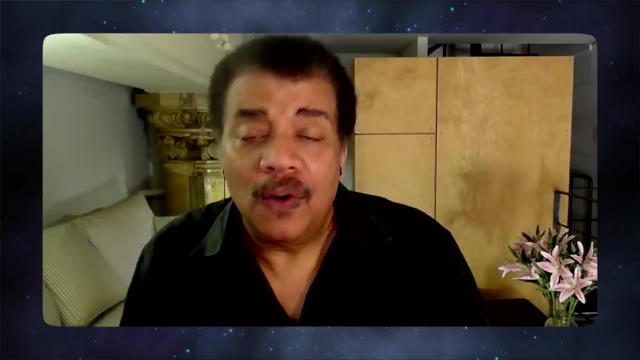 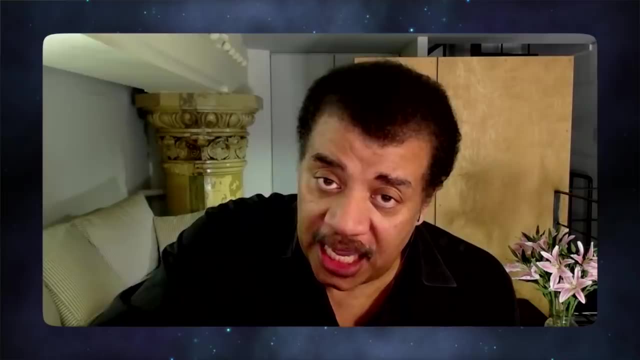 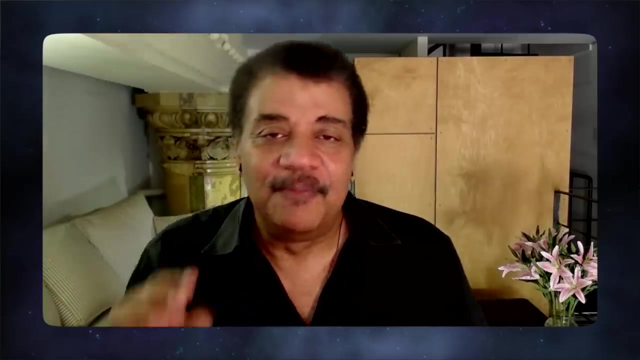 that is the temperature of the Sun, and so so, when daylight does that look blue, do you know? I mean, but it's bluer than a, than a cooler, well, cooler lamp, check, it's a low-temperature lamp, right, but but if you look at the 5600, that's. 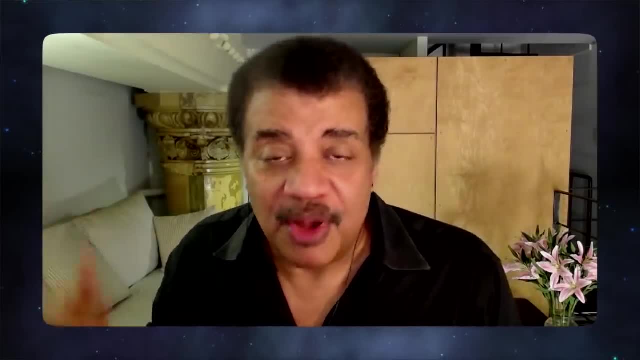 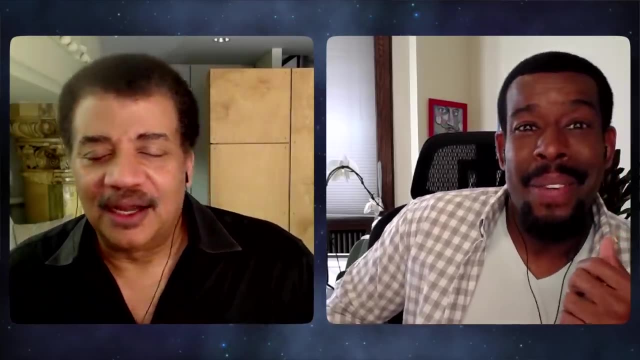 daylight. by the way, it's not yellow, that is not a yellow lamp. yet you still have people saying the Sun is yellow. so no, it's not. the Sun is freaking white. okay, right, I interrupted you. I mean, that's that you? basically that's what it is, but 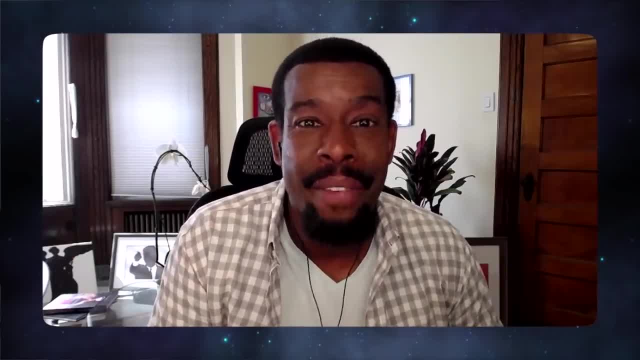 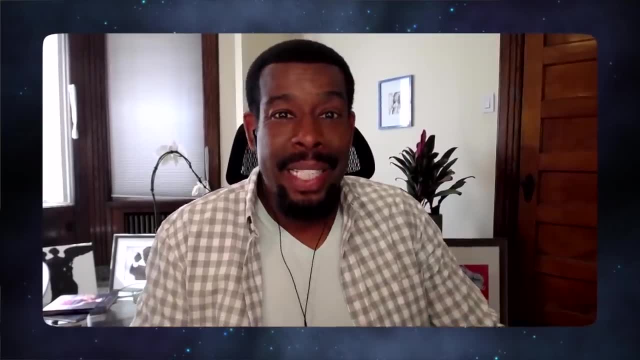 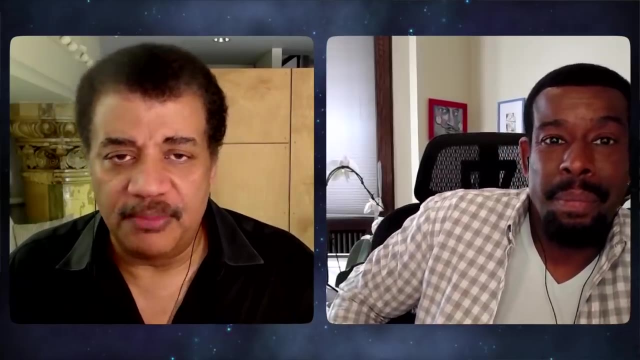 that it's really like the only reference that photographers have. but what you're saying is: photographers need to come up with a new reference, because what they're saying is scientifically wrong. the numbers are. it's artistically sensible, but then don't put numbers on it, because with these numbers mean things. are you gonna put it 10,000? 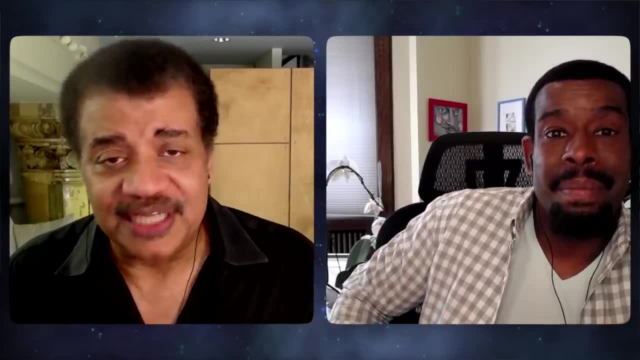 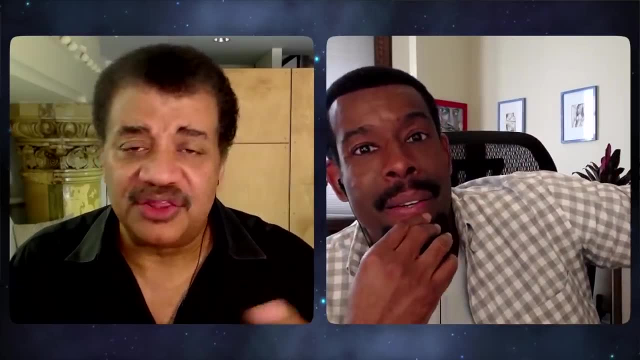 degree lamp. that's a hot lamp and that's a very blue lamp. blue is hot in the universe. that makes sense. I mean, now do we have blue stars? They're 20,, 30,000 frickin' degrees. We have red stars. 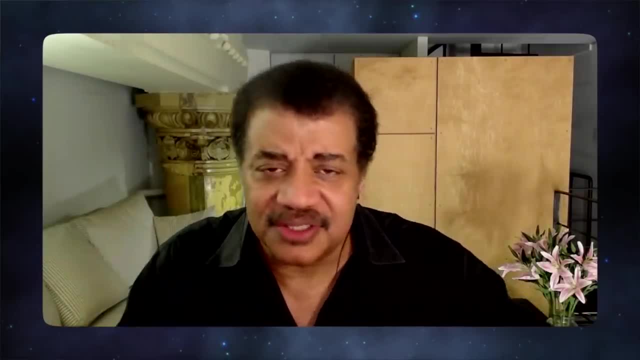 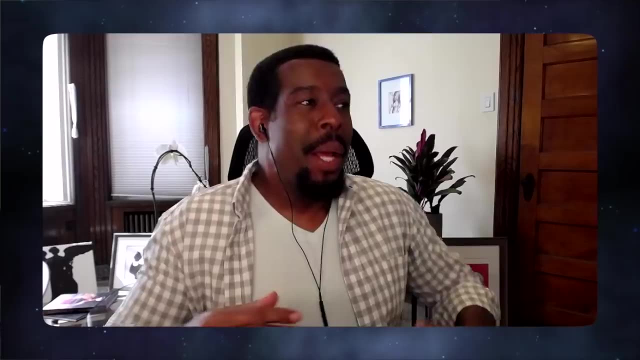 They're called red giants. They're hovering around 1,000, 1,500, 2,000 degrees, Barely glowing. So I'm, I'm, I don't know. I like what you're saying. I just like the fact that I'm changing red hot to white hot from now on. 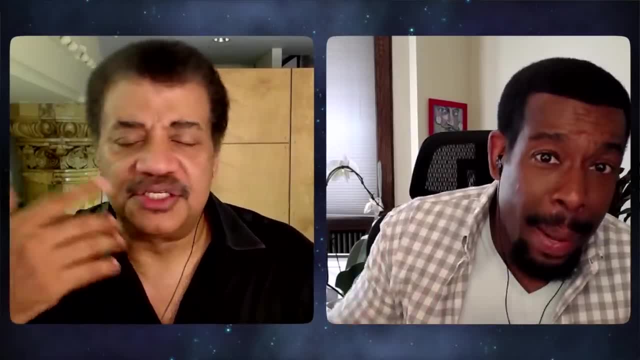 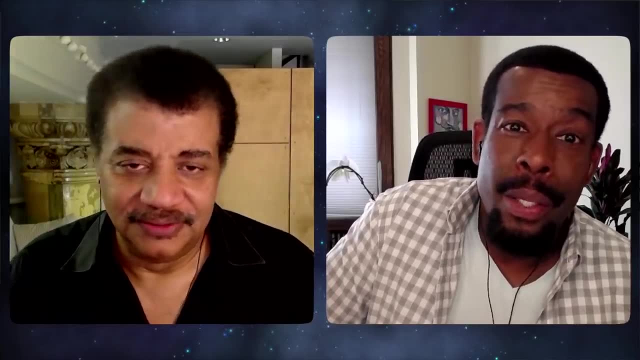 Now some people know that white hot is hotter than red hot. Right, It's just not common in society. But blue hot is my newest thing. I'm going blue hot all the time. You know what I mean, Don't you know what? 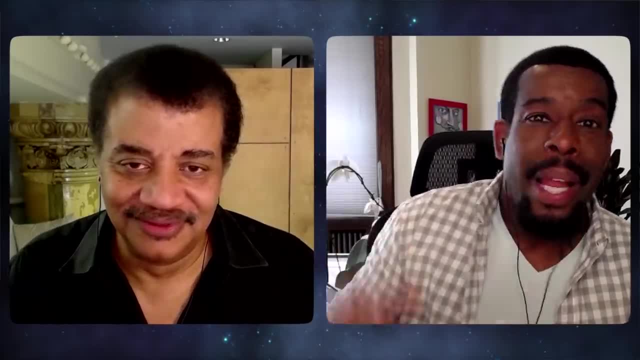 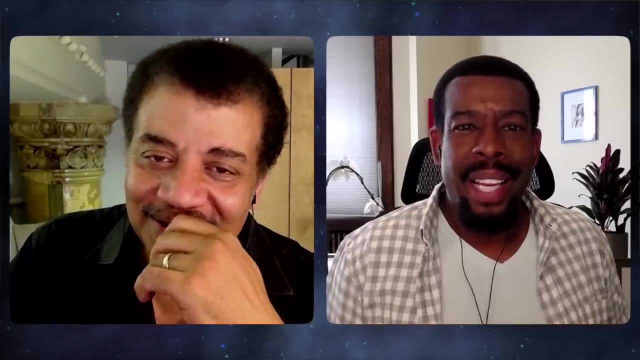 All the way with a blue hot poker. That's what I want for you. Oh no, The problem is it's melted. by then, I mean a fireplace poker. That's a problem. That's right, You're right, Because it's oh yeah, that would melt. 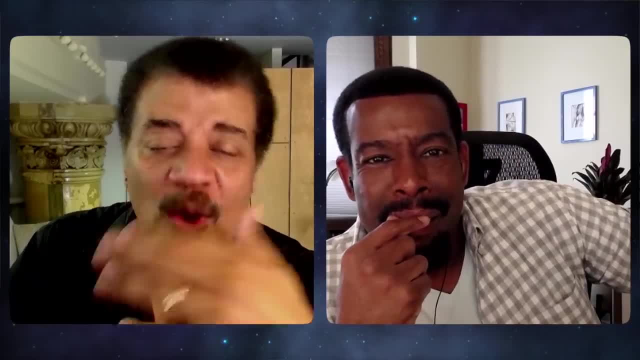 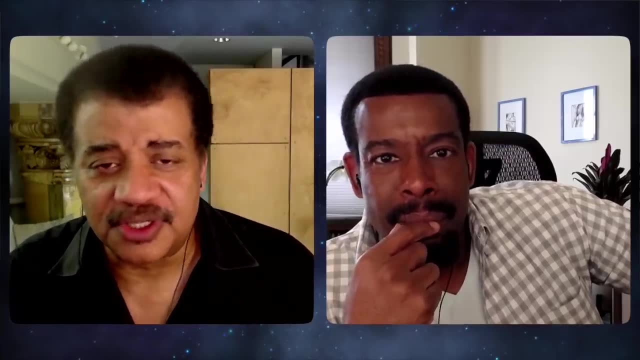 Damn. Yeah, yeah, yeah, You start melting stuff. That's a problem. That's why we have very little experience with white hot and blue hot. But red hot you can get almost anything to red hot temperatures. Yeah, you don't see a lot of white. 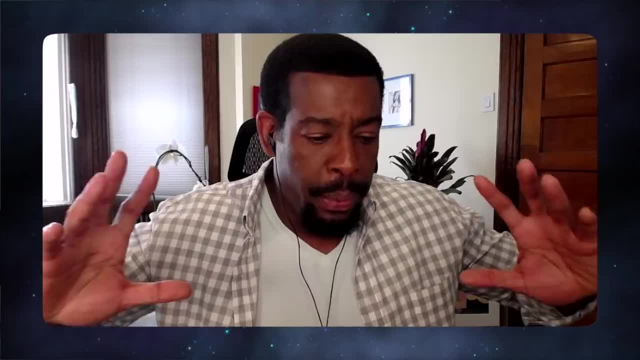 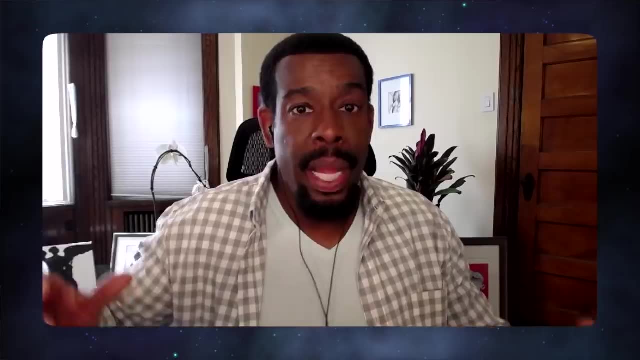 You don't see a lot of white hot, though. No, you don't. You know, my dad was a printer And so, in printing, he owned a printing company, And the coolest thing in the plant was how you make photo plates. 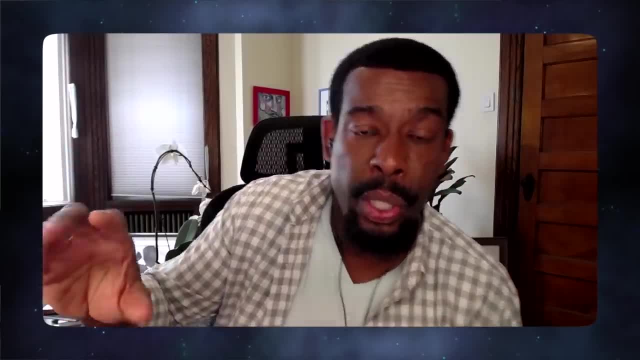 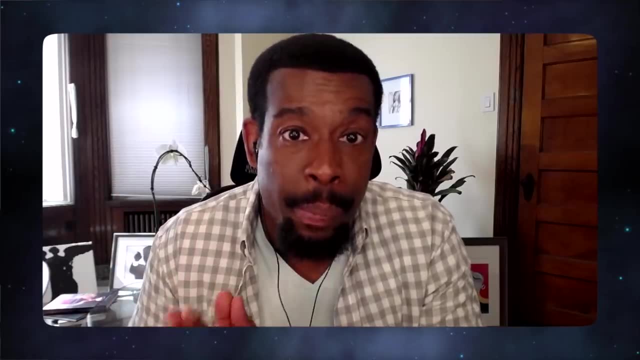 So the plate is treated with a chemical that, when exposed to this super white hot light, the image is burned onto the plate And it's called burning a plate Right, And then that image is the only thing on the plate now that will transfer ink. 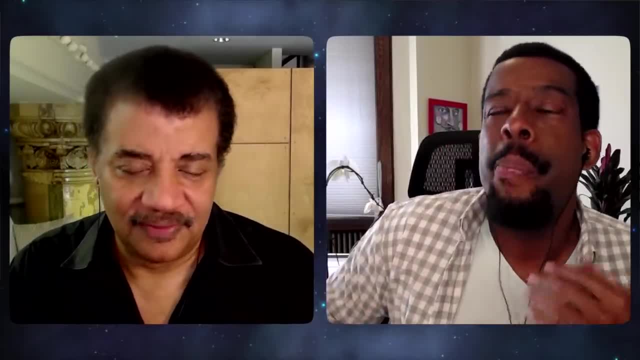 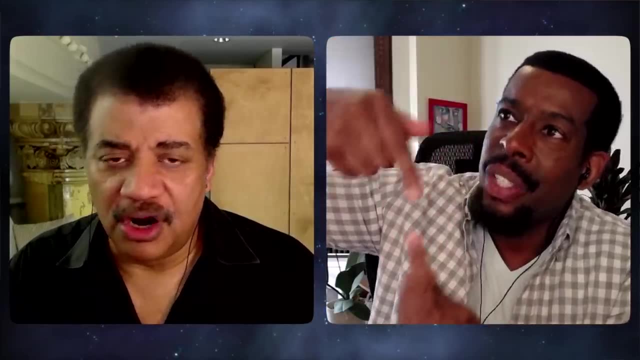 And that's how you transfer an image. But they used, I forget the name of these little tubes. They came together and they and I forget- Oh, it's an arc, lamp Arc. yes, Yeah, yeah, carbon arc. 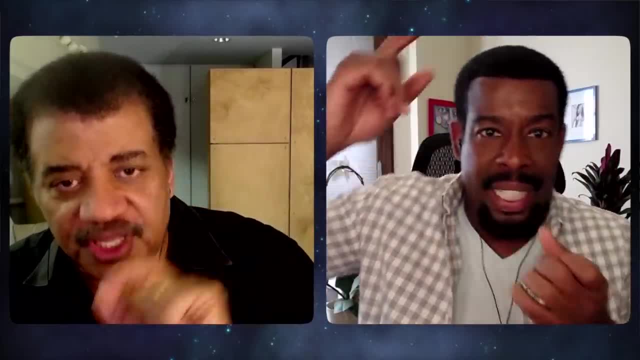 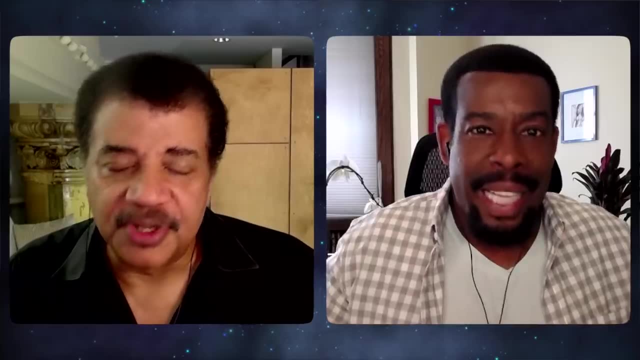 And the light in between. That's a very high temperature arc between there. That's correct, And it was the coolest thing in the world And you weren't allowed to look at it because it would make you blind. Right, because it's high in ultraviolet light. 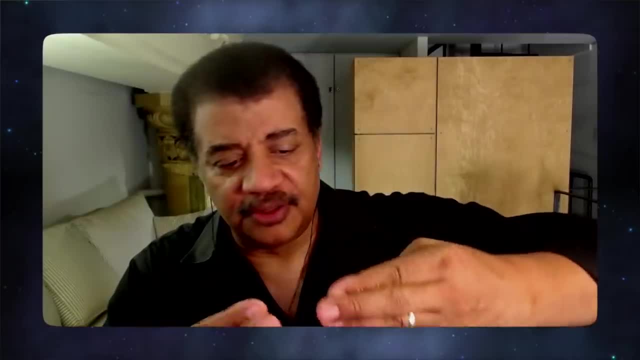 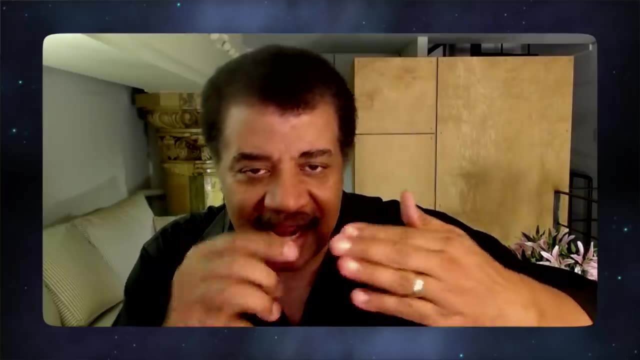 It's very high energy light Right, And what they do is they have these carbon Carbon rods, basically, And you you attempt to send current through it, but it has to gap across an air gap Right, And depending on what your separation was and how big your current was. 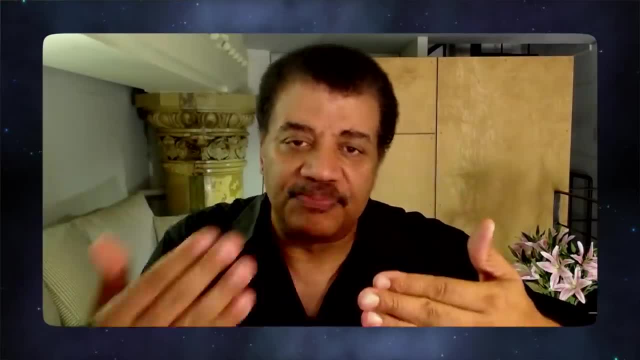 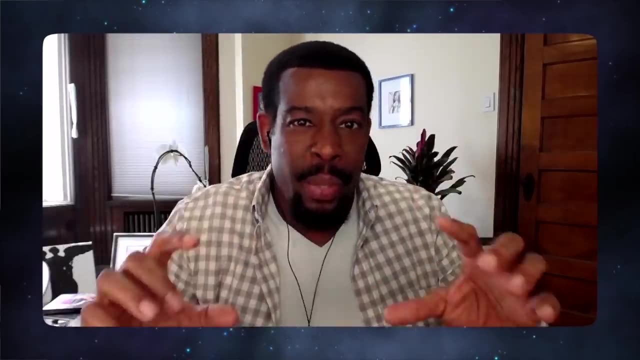 you could determine how, what the threshold was before you jumped the arc Right And there, there it was. That's exactly it, And the whole thing was just those two tubes and the light in between, And you had to look at it with like the same way you look at- I forget the glass. 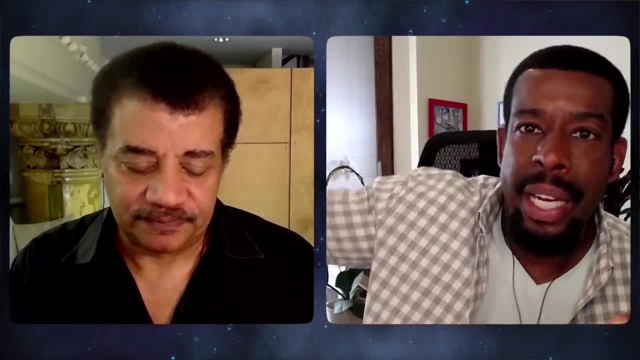 The welder's goggles. Yeah, yeah, It's a welder's goggles. You got to look at it. with that Same thing, you look at an eclipse with Mm-hmm, mm-hmm And it was the. it was the coolest thing in the world, but it was white hot. 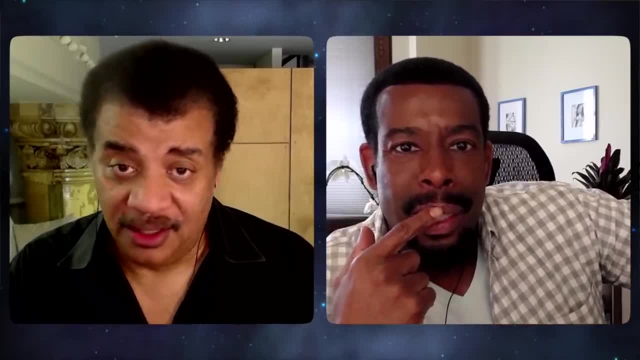 Yeah, yeah, And and and hot, very clearly hotter than anything. red hot, Right, Yeah, That's what that is. So I, so these are my issues that I'm bringing to you, Chuck. I don't have a solution for them. 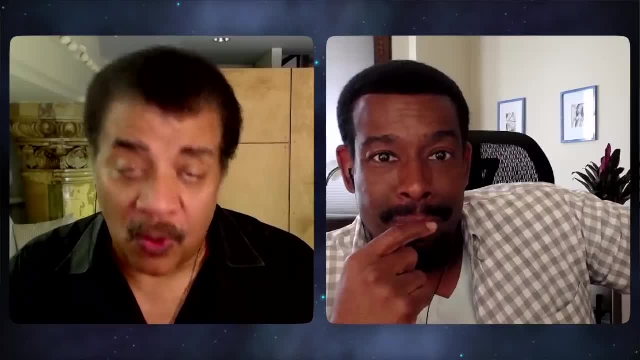 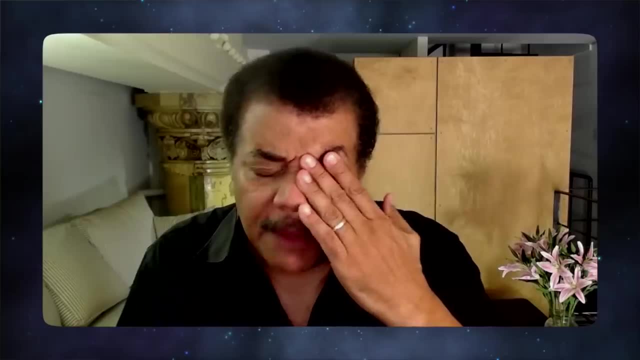 I'm just highlighting them. And and, by the way, when I walk up to a water cooler, and, and one and the, the, the two spigots are color coded. Yes, One is red And I say, okay, I'm no longer in my lab. 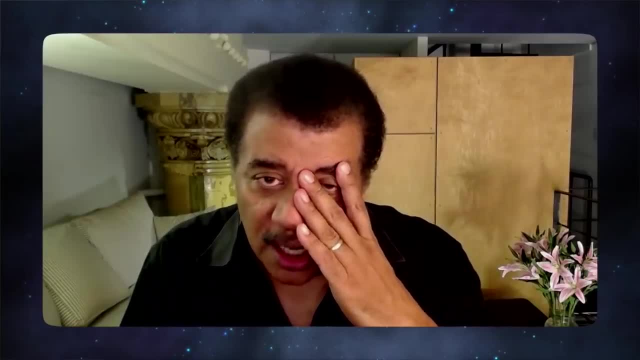 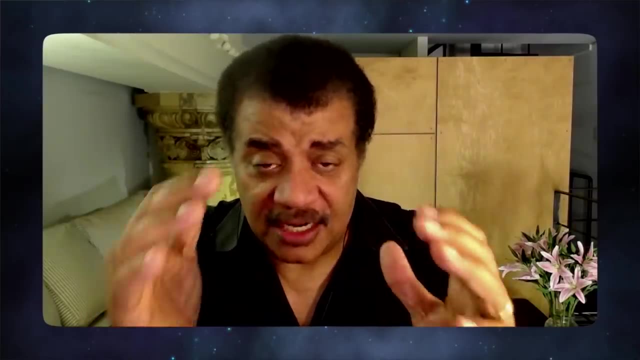 I'm in the real world, And so blue is not Hotter than red. They think blue is cold. So that's my I. I waste. I can't tell you how much of my life I've wasted staring at twin spigots on a water cooler, figuring out which one is the cold water. 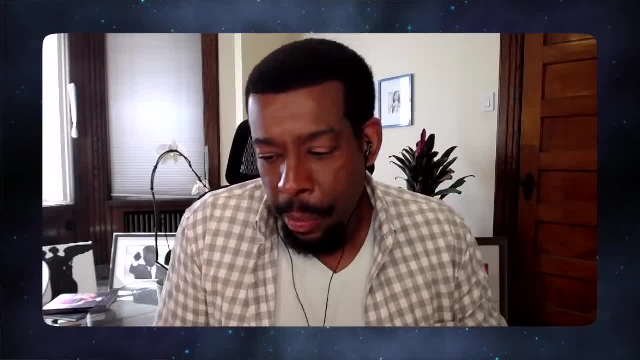 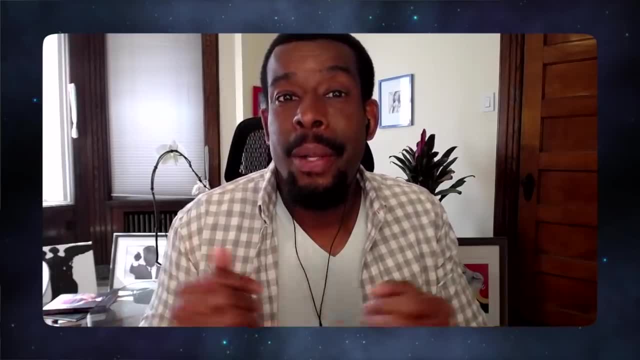 Well, so what we should do is maybe the red is hot and then maybe pink for, like, the cooler blue, for the cooler water, Like you want the water. Keep working on that, Chuck. I don't know about that. Keep working, Oh great. 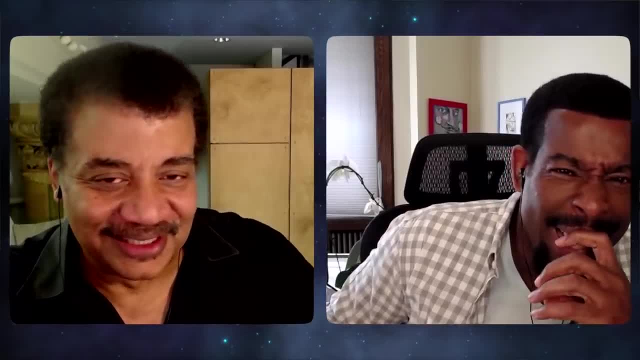 Great. No, nobody wants to Drink gray water, That's for sure. I'm trying to. All right, That's all. That's the. that's all I want to do on this explainer. That's a really cool. 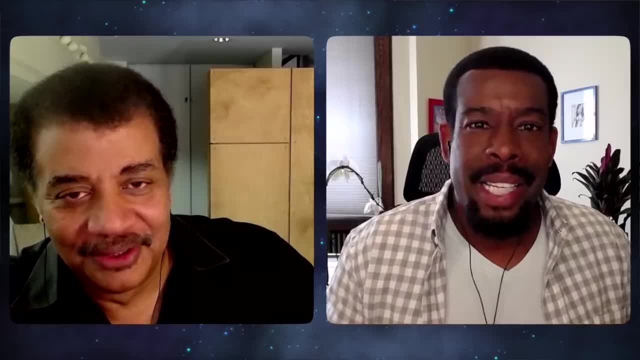 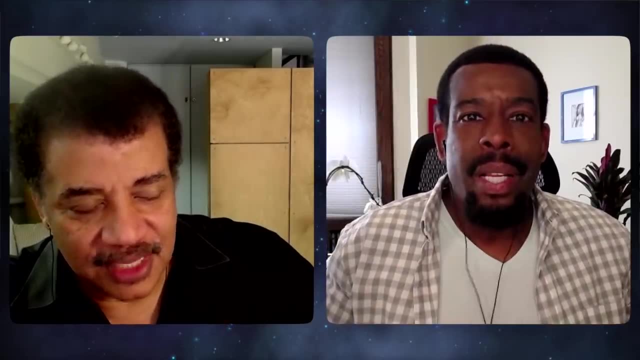 But see, now you got me mad at the fact that all these things exist in life that tell us that blue is cooler than red Cause now that you said that it's everywhere, And even the photographers know it's hotter because they ask for a higher temperature. 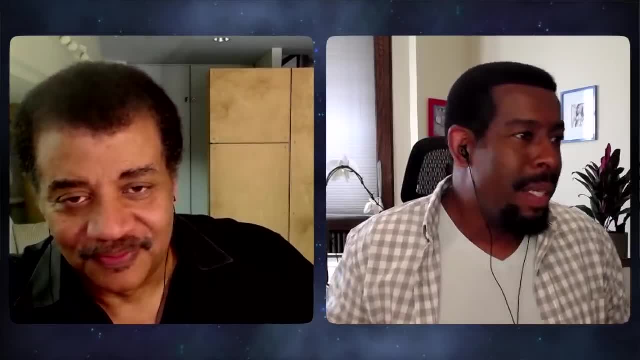 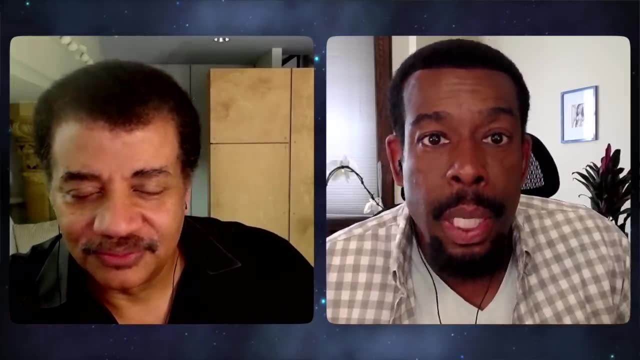 That's right, That's that's. that's the insidiousness of it all. All right, Cool. Anyhow, I know what we should do. Here's the solution: Next time you see a Photographer people, Just punch them. 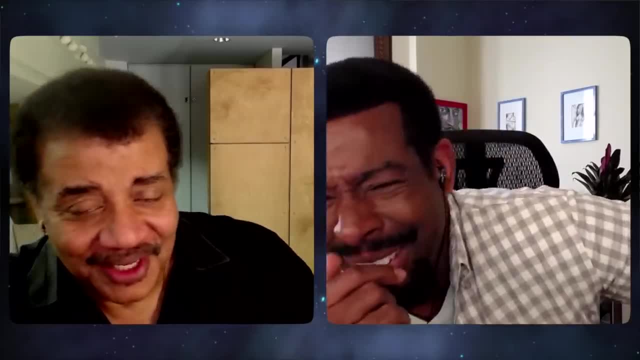 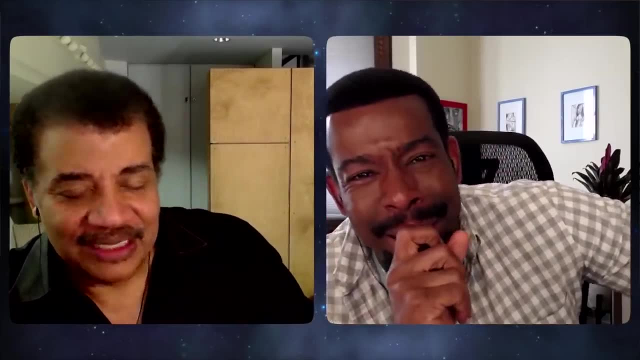 Did that work for you so far? Is that really? Is that how you? you did that to your boss a few times. How far did that get you? No, Exactly, Did we find you on the street before you had this gig? 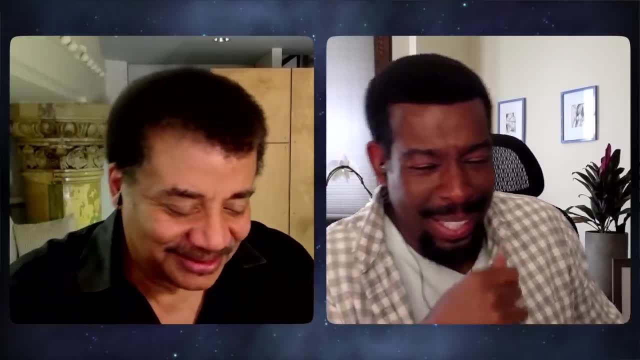 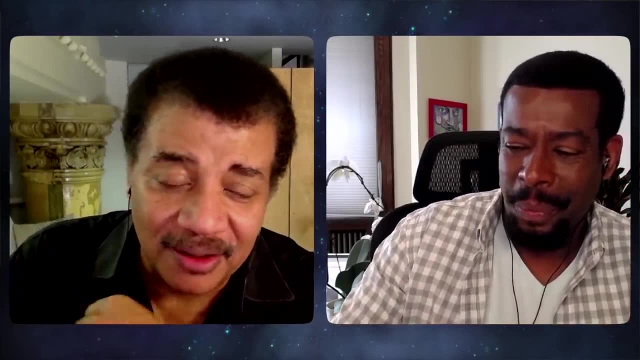 Right, I punched my boss one too many times, Exactly. All right, dude, We got to go to quit it there, All right. Thanks, Chuck. This has been a star talk and explainer On the temperature and color of light and the fight between the astrophysicist, the 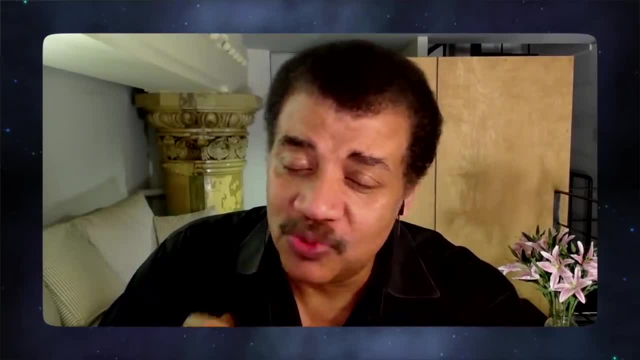 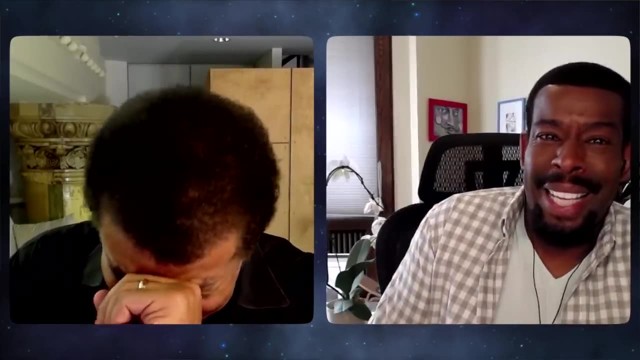 artists and the photographers, And we, the astrophysicist, will probably lose. but that's okay, There's other fish to fry out there, Not if you punch them. Sneak that in and low point, Go ahead, Go ahead. 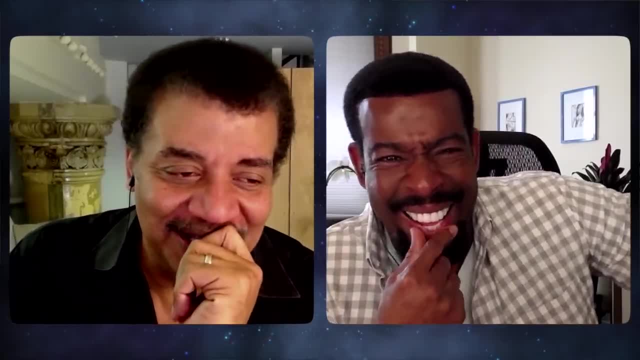 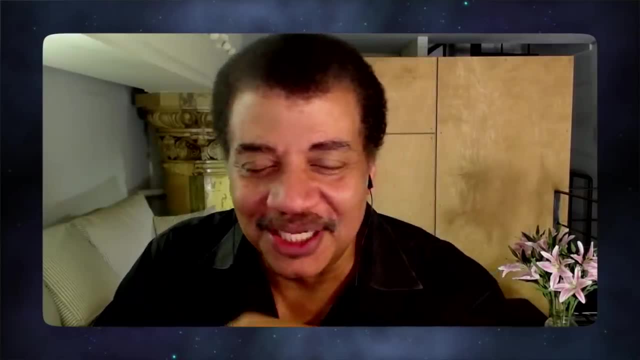 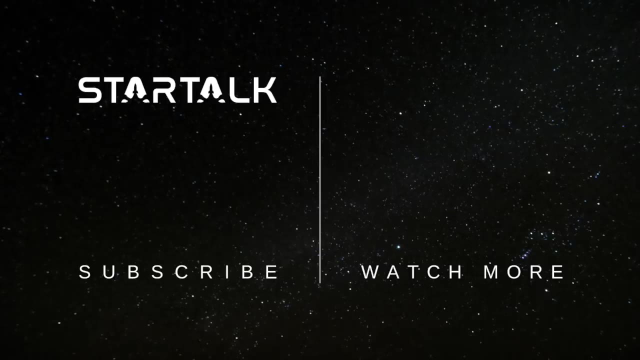 You get your way real fast, Neil. Just punch them. Oh, Oh, All right, The star talk explainer, Neil deGrasse Tyson, Keep working up. Bye, Bye, Bye, Bye, Bye, Bye, Bye.